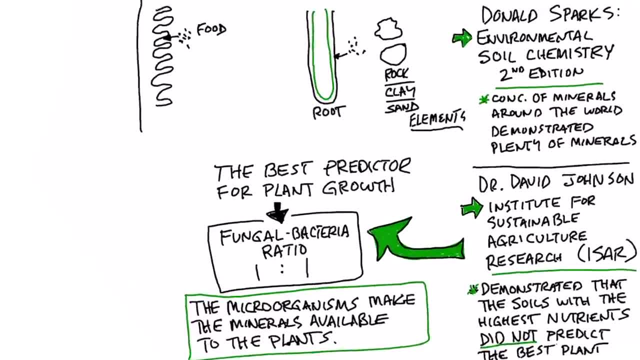 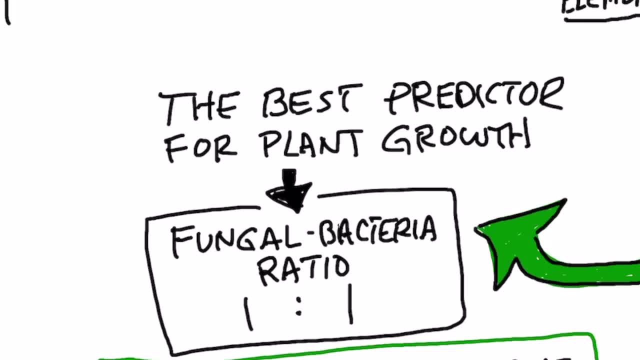 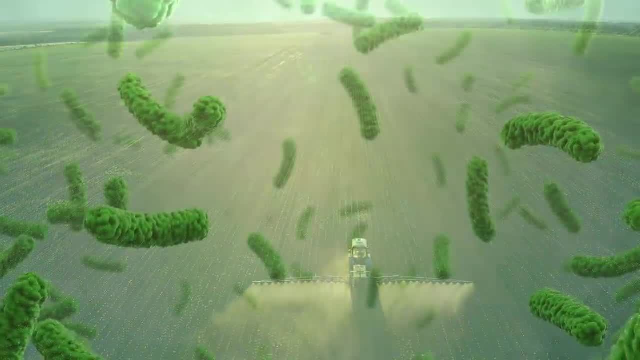 which will explain everything, is this: The best predictor of plant growth and plant health was the fungal and bacteria ratio. You see, as you use the farm and you use pesticides and insecticides, what happens over time is you lose the fungal growth. 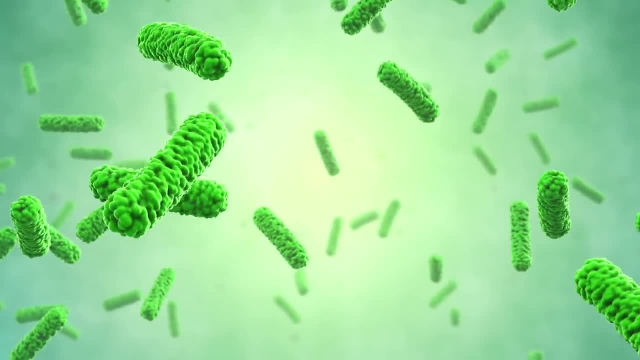 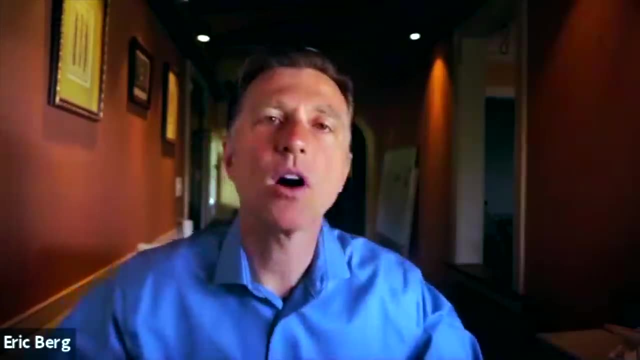 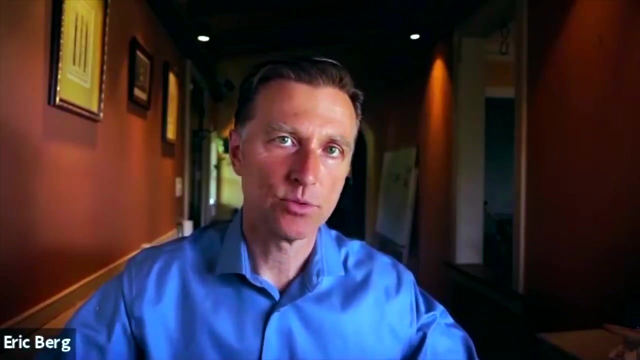 until your bacterial counts become higher and higher and higher, to the point where you're 100% bacteria and no fungal. You see, fungus is a very important part of soil. It's part of the microbial flora that helps break down the rocks, the sand and the organic material. 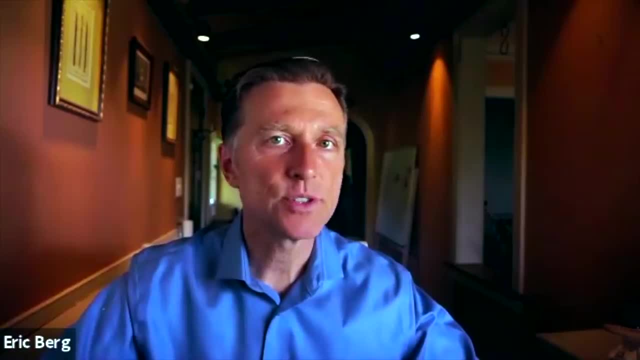 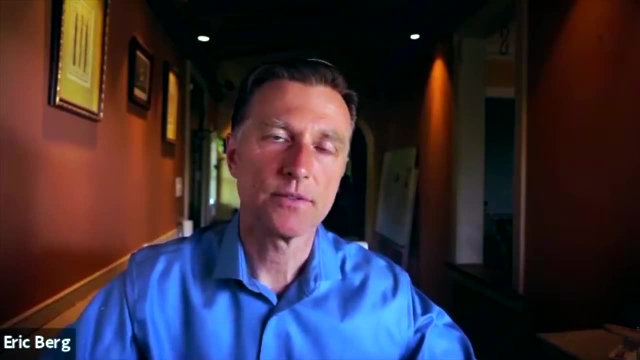 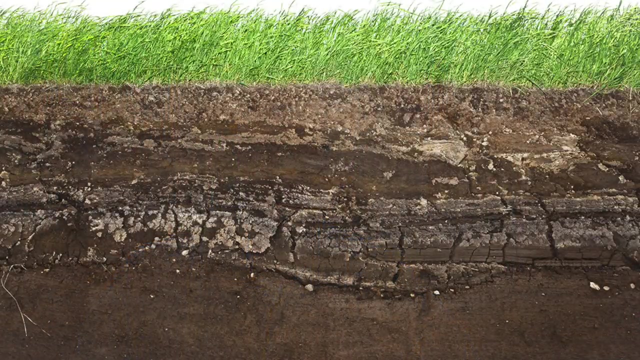 and then makes the Minerals available to the plant. It's both the fungus and bacteria that make minerals soluble for the plant so it can be usable and exchangeable. And without those microorganisms the minerals basically are locked up in the clay, in the sand and the rocks. They're unavailable. 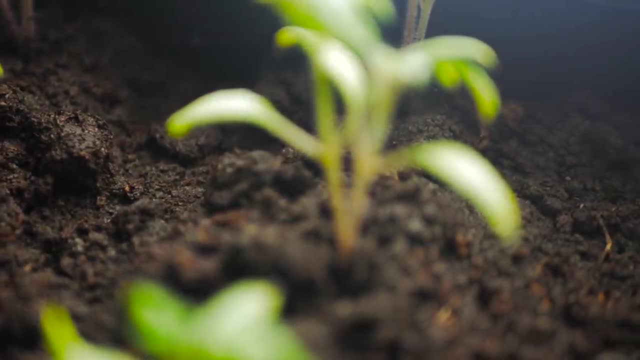 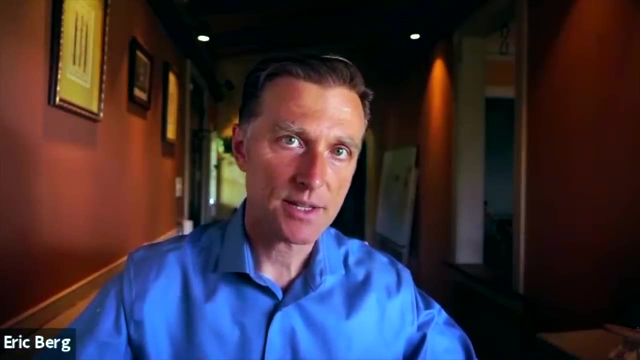 to the plant And you need a ratio of one-to-one fungus to bacteria And this is why a lot of farmers have to use MPK- the 19th century- And they're not going to be able to use MPK phosphorus and potassium, because they can just give the plants some quick nutrients to get them. 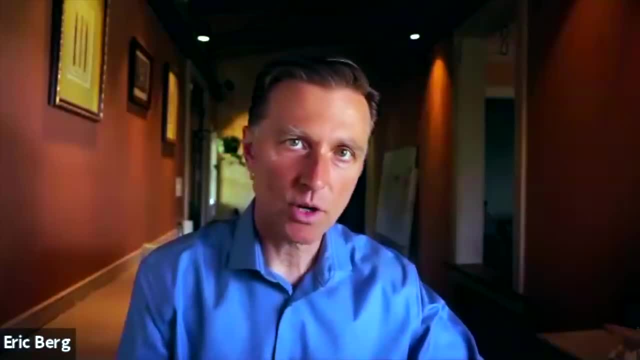 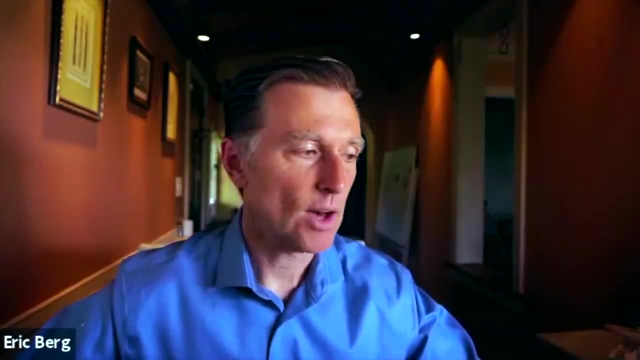 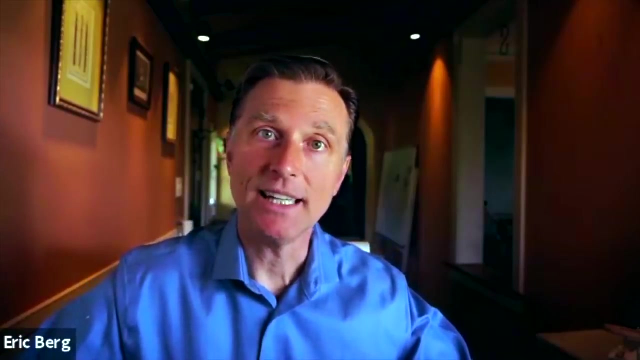 to grow because there's very little microbial growth. that is making the rocks available for that plant. Now, how does this relate to our bodies? Well, we need microorganisms in our gut to assimilate food. We need acid in our stomach to actually 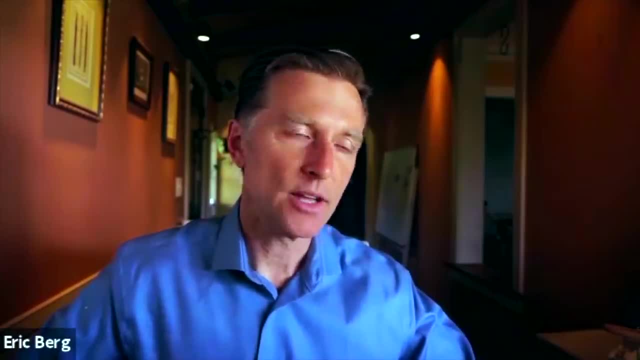 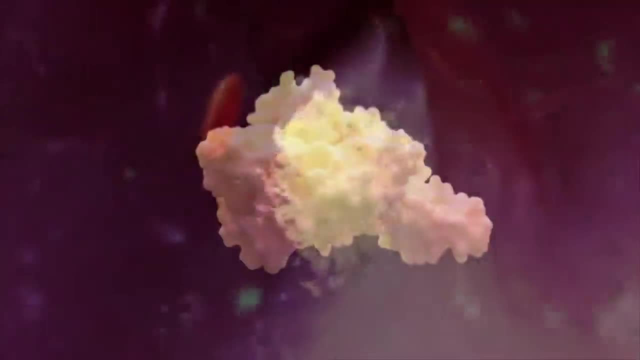 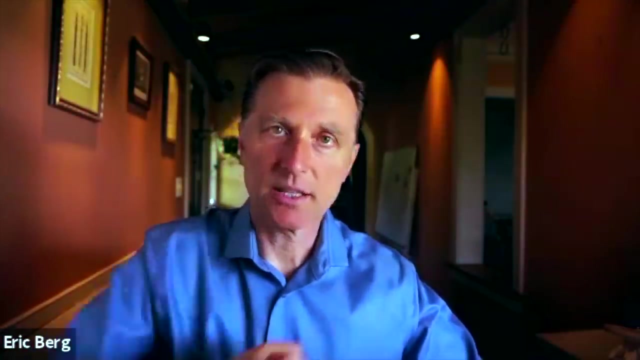 Help absorb the nutrients from the food to break down the proteins. Without the acid, we can't absorb minerals We can't break down protein into amino acids. Without bile salts, we can't extract fat-soluble vitamins. Without enzymes, we can't break down the food to extract. 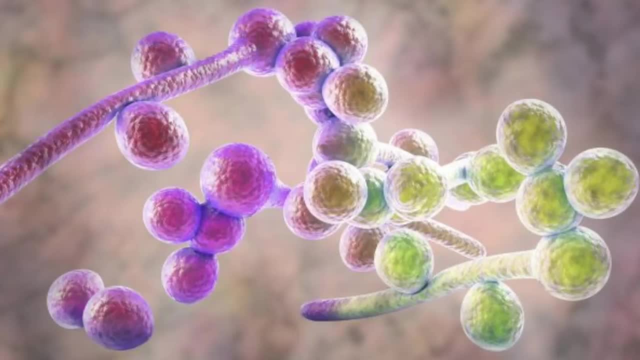 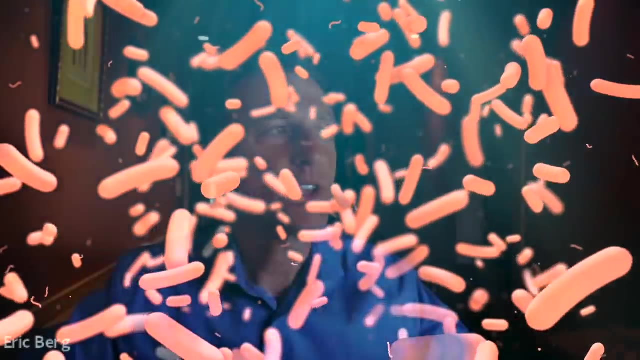 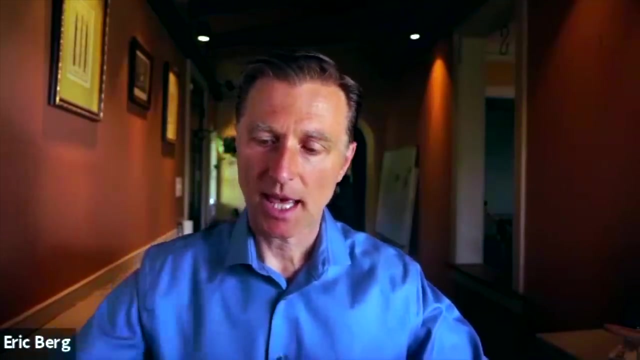 the micronutrients, And without friendly fungus and friendly bacteria we can't actually break down the food either to extract nutrients into our body, And so a big mistake that people make is they go to the store, they buy their one-a-day vitamin and they're buying.